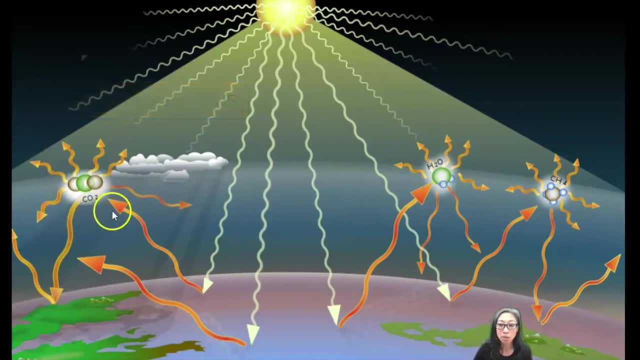 in the atmosphere. So this responds in a specific way based on the shape of the molecule. Same with water. This also, when hit with infrared, responds. And methane- This also responds when hit with infrared. Infrared energy will cause this bond to vibrate or 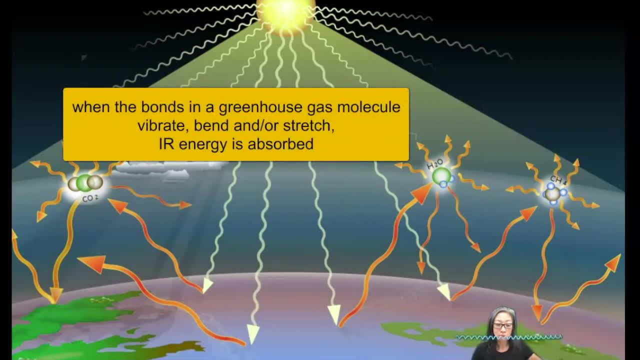 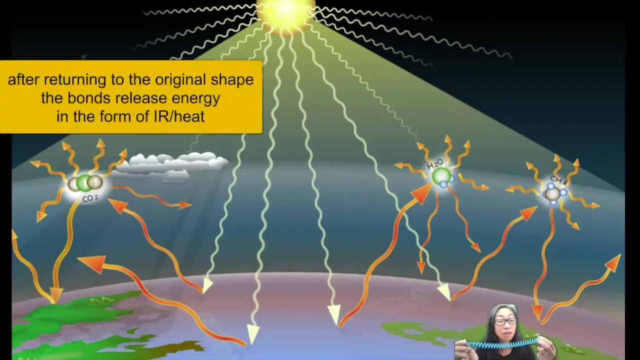 bend and stretch. Energy is absorbed. When the molecule bends or stretches, it holds that energy like a spring, but also like a stretched spring. This spring will eventually release And when it releases, the energy that was there is released into the atmosphere as heat. So that's what we can see here. is that the carbon dioxide molecule 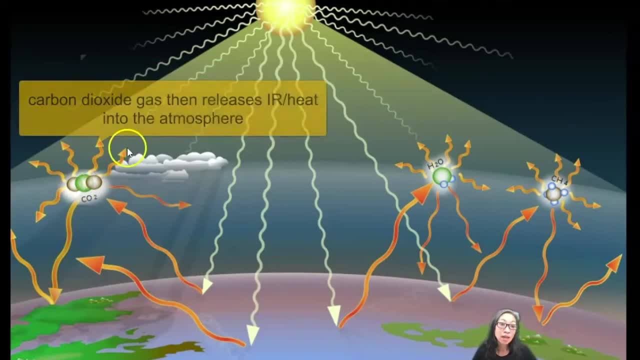 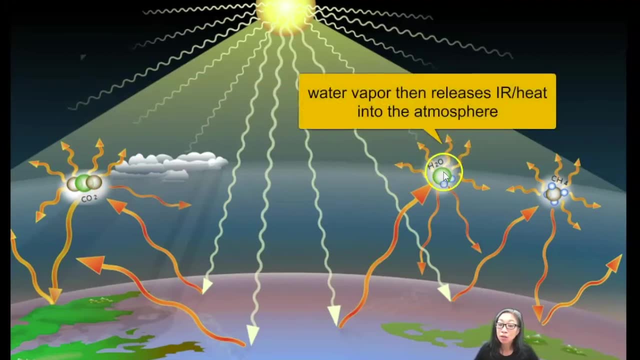 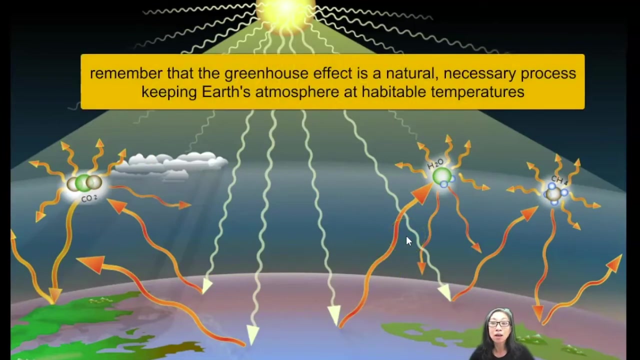 absorbed infrared and then releases that energy as infrared heat. Same with the water: This absorbs infrared and then releases infrared, So that's infrared that is released and the process is the the trapping of heat by these molecules into the atmosphere before the infrared can be released out to outer space. 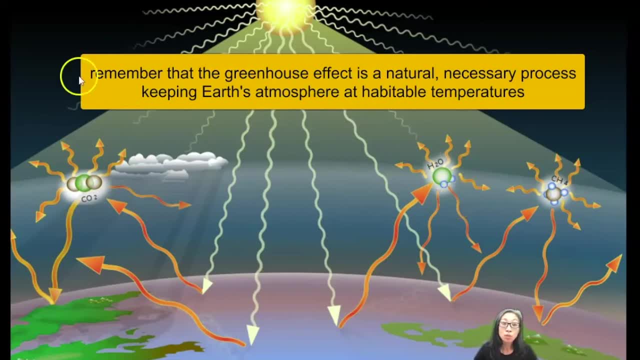 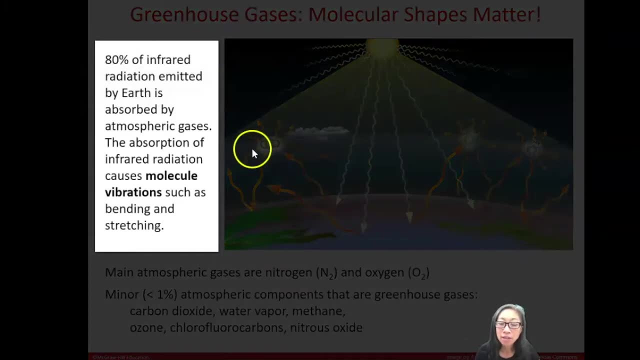 So this allows some of the radiation that would be released to remain in Earth's atmosphere. This is the process of trapping heat in the atmosphere. You have these gases in the atmosphere, they have specific shapes and the bonds in these shapes will absorb infrared. 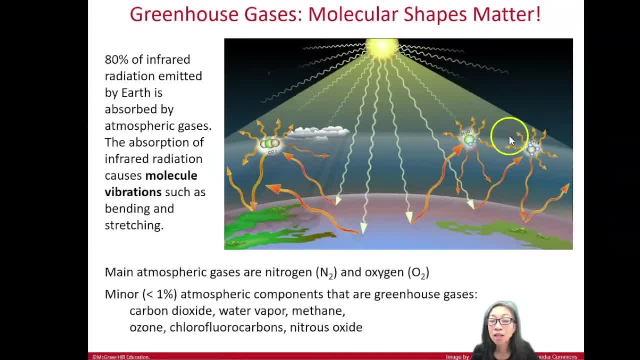 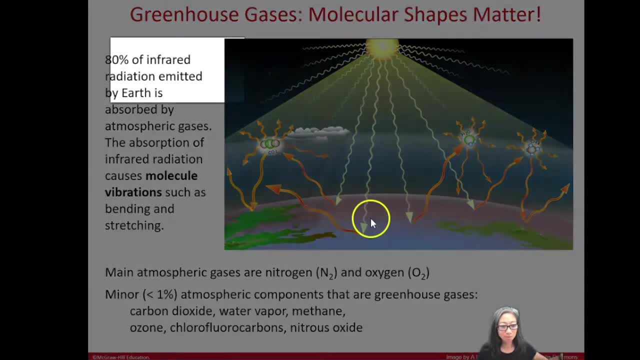 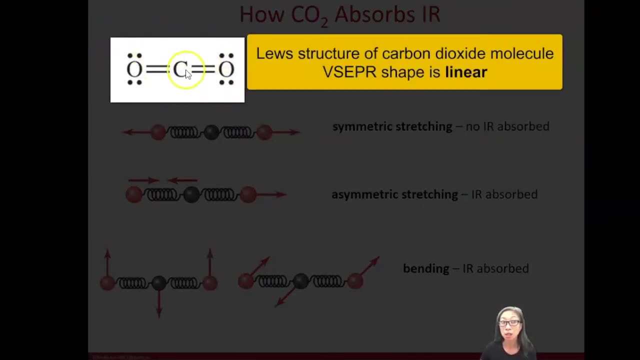 and then release infrared, keeping the infrared in the atmosphere before that infrared energy can be released or escape or emitted out to space. This is the Lewis structure of the carbon dioxide molecule and the three-dimensional shape is linear. There's a central atom with a bond on either side. 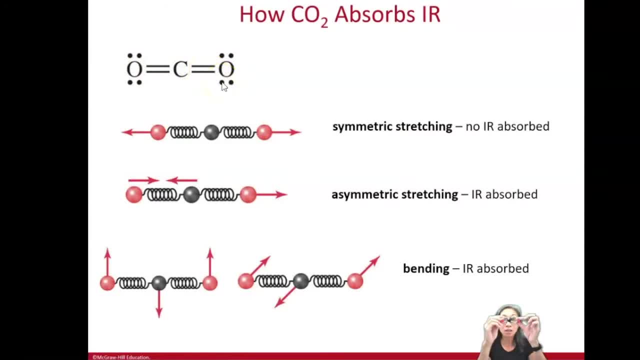 This is a double bond, and this is a double bond, And so this is the linear shape It has. the central atom is shown as this carbon, which is black- Carbons are typically black- and then the two oxygens are the red atoms. 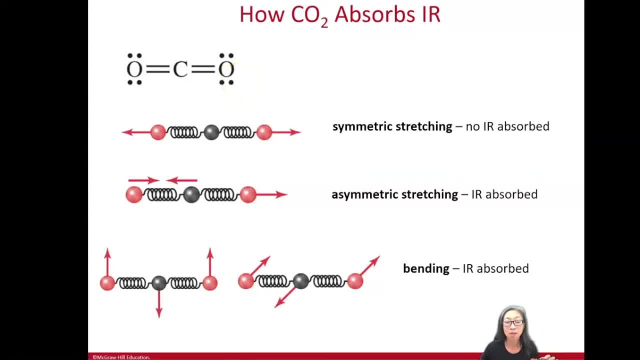 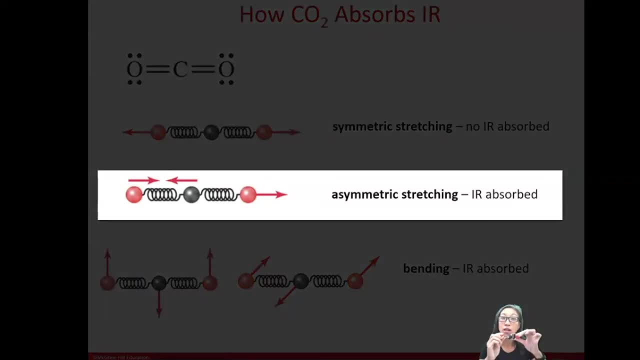 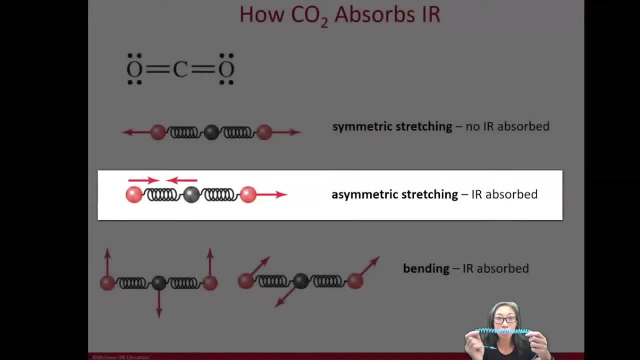 So there's stretching and there's bending, But at another level there's symmetric stretching and there's asymmetric stretching. This asymmetric stretching absorbs infrared. So this absorbs infrared temporarily in the bonds and when this returns, this will release the infrared to the atmosphere. 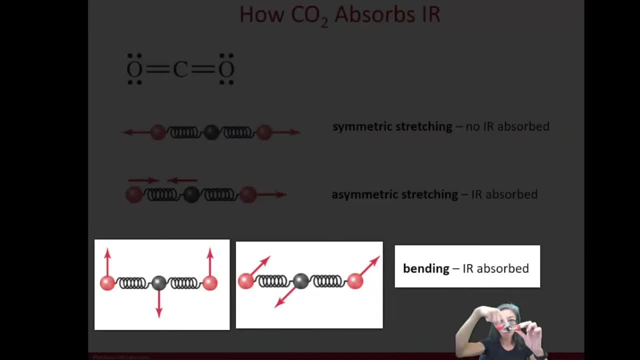 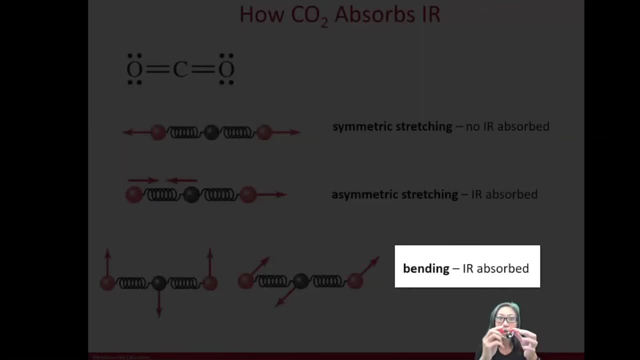 With bending, this molecule infrared hits this and then this can bend like this. When this bending happens, this causes the entire molecule to have this overall kind of V shape. Well, this is not the natural shape and it is also causing the two oxygen atoms. 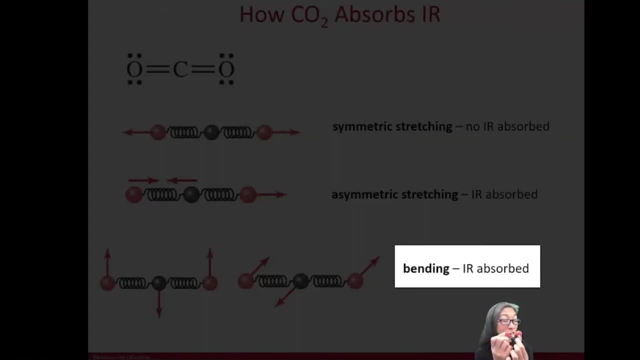 to be closer together and the electrons on those oxygens don't want to be close together. Remember: the reason why this is a linear shape in the first place is because the electrons want to be as far apart as possible. That's VSEPR theory. 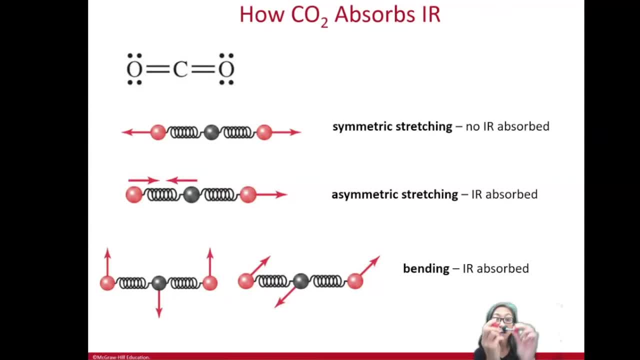 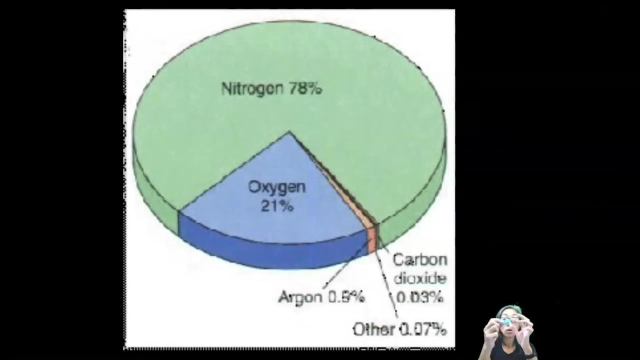 This is a temporary shape, and then the molecule will return Back to its linear shape. When this returns back to the linear shape, the infrared energy that was absorbed then is released. The main atmospheric gases are nitrogen. This is N2.. It's two atoms bonded together. 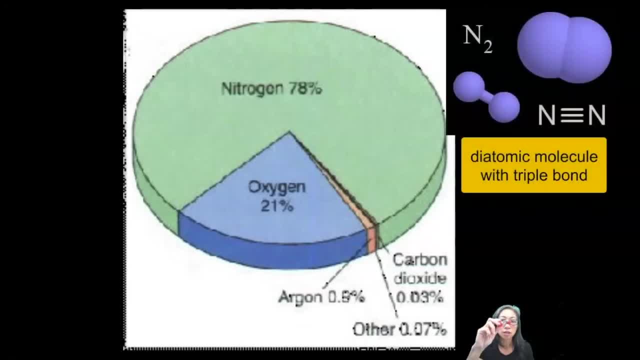 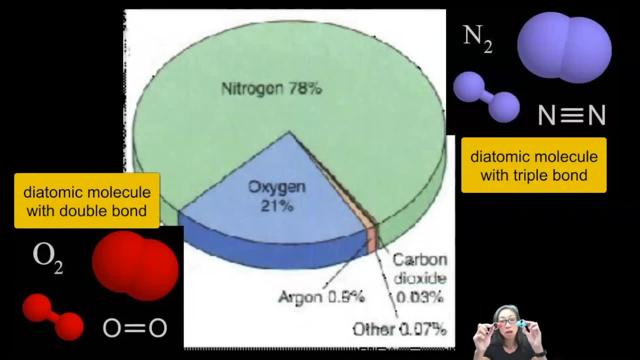 and that's a triple bond there, And also oxygen. This is O2.. That's two oxygen atoms and that's a double bond there. But you can see, these are simple molecules and these are not greenhouse gases, because they really don't absorb anything. 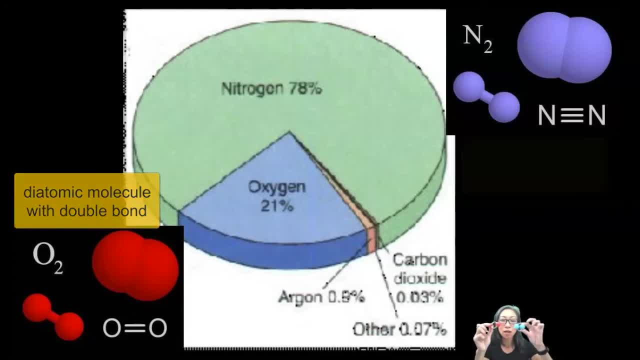 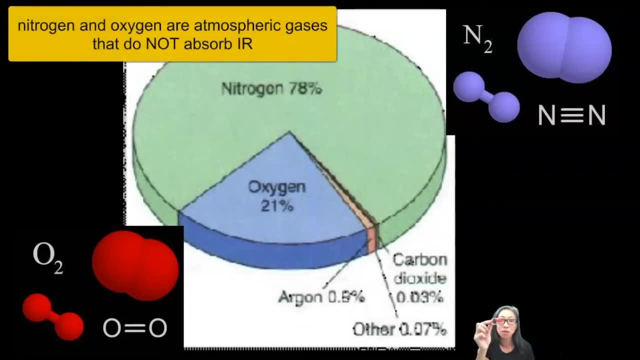 They don't absorb anything. They absorb infrared by bending or stretching. They can vibrate a little bit when absorbing infrared, but this does not cause any bending or stretching, It just causes a little bit of molecular vibration, and so infrared does not affect these nitrogen. 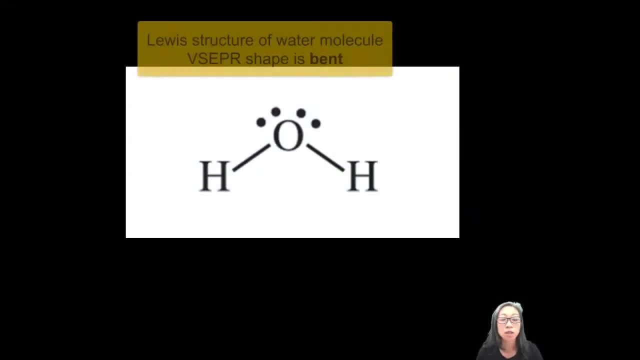 or oxygen molecules, and they don't trap heat as a result. This is the Lewis structure of the water molecule. It has the bent VSEPR shape. There's on the central atom this oxygen. There's two bonds and two lone pairs, So that's bent. 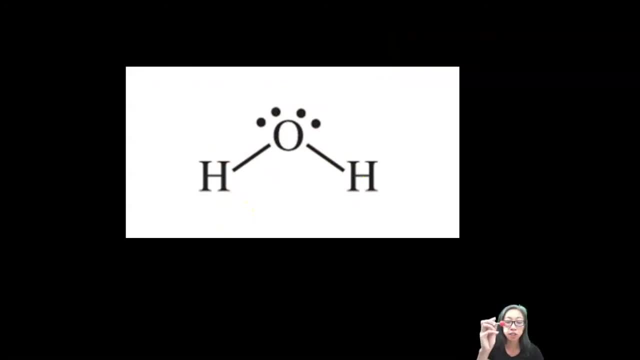 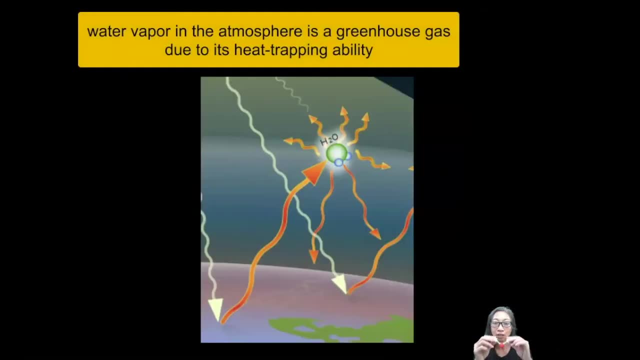 Instead of linear, The bent shape is a V shape and this is water vapor in the atmosphere and is also a greenhouse gas similar to carbon dioxide. When infrared hits this, it will bend and temporarily absorb the infrared and release back to its less bent shape. 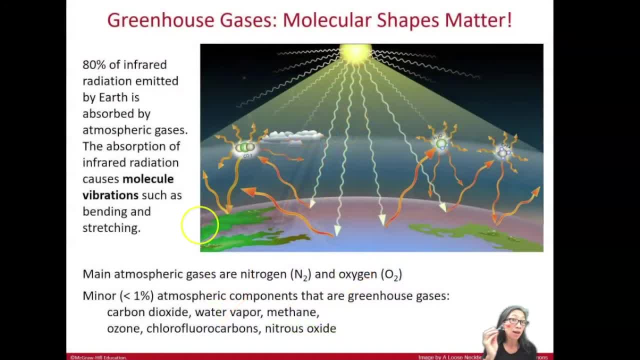 and release the infrared into the atmosphere as heat. As there are more and more carbon dioxide molecules, more and more infrared will be absorbed and more and more heat will be trapped, and so that's what's going on in the process of global warming.